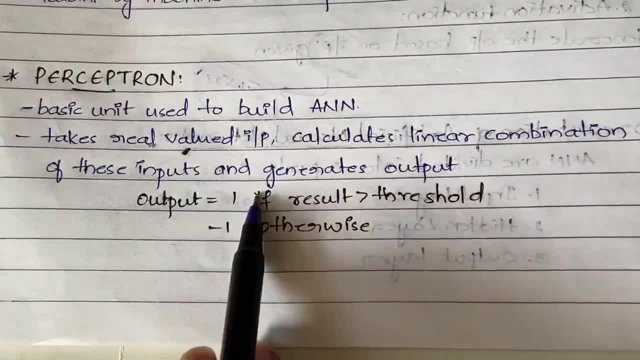 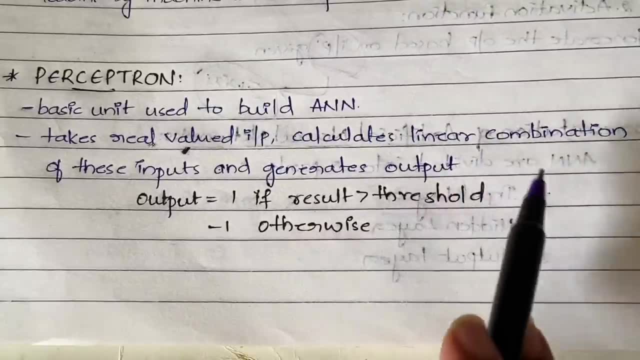 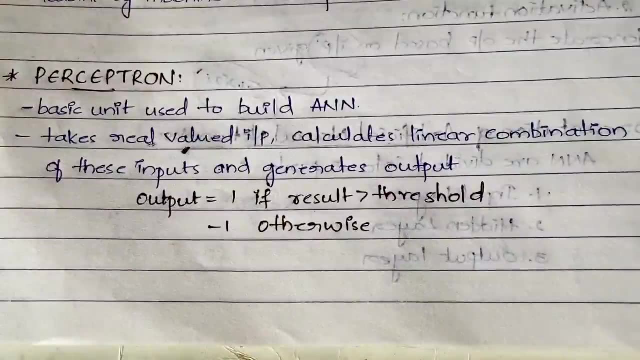 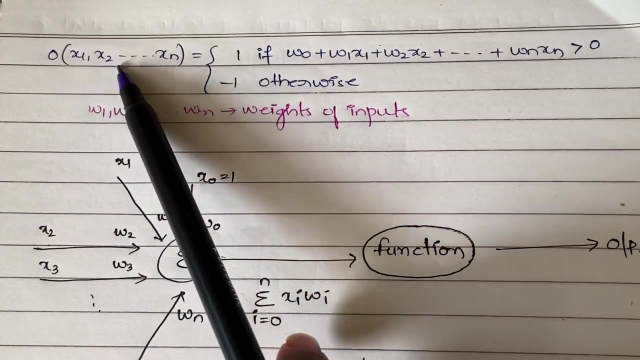 If, sorry, the output will be equal to one if the obtained result is greater than the threshold value. Okay. it will produce negative one if the obtained result is not greater than the threshold value. Okay, done So. this is how a perceptron works. and let us see what is linear combination. and you know the perceptron training rule as well, right? So yeah, if you can see this O of X1,, X2, X and so on, O is nothing but output: output of X1,, X2 and so on. 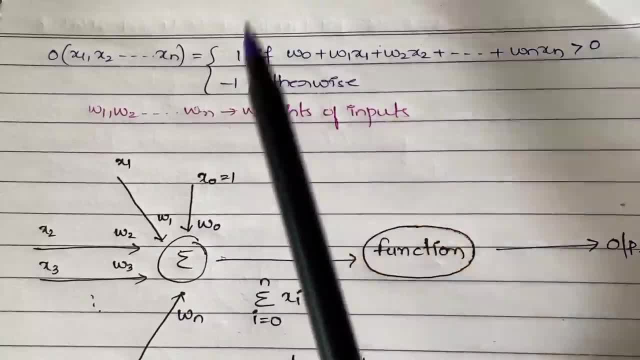 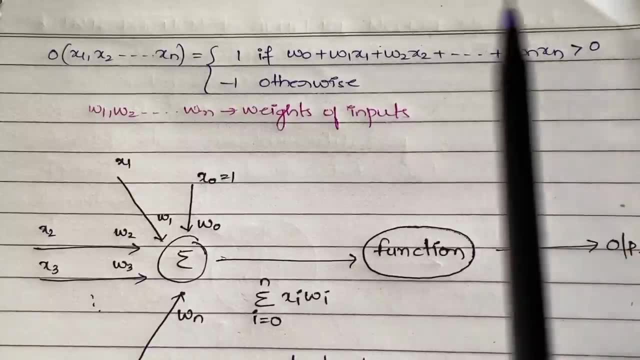 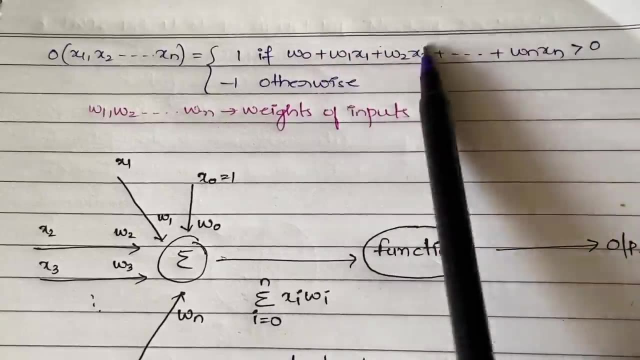 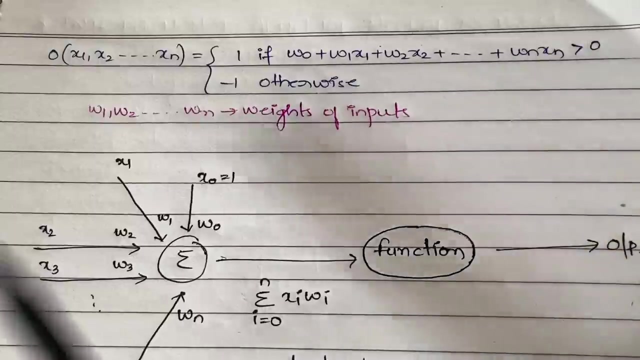 Up to Xn will be equal to one or negative one. One when W0 plus W1X1 plus W2X2, and so on, up to W1Xn is greater than zero. If it is not greater than zero, it will be negative one. Okay, and what is this? W1, W0 plus W1X1, and so on, This is the linear combination of the inputs. W0 is the initial weight, Okay, and W1X1, W2X2 are the inputs and their corresponding weights. Okay, so I will tell you now how perceptron training works. 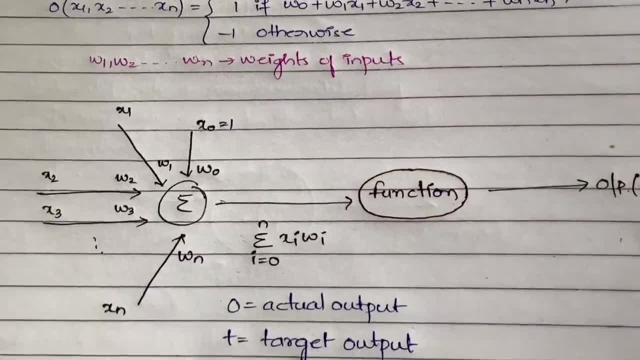 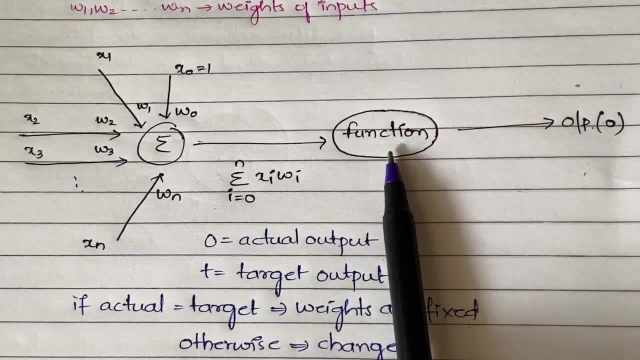 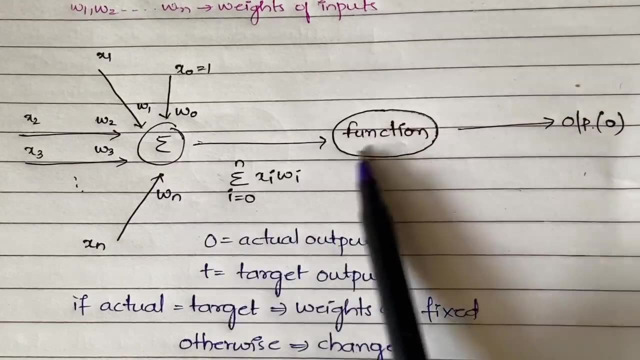 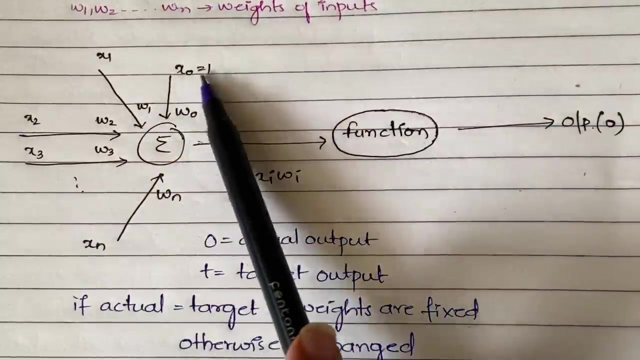 Rule will go on. that is how we will be training our perceptron, how we will be taking our input values or output values, right. So first see, this is a summation and this is the activation function. right, A node has two paths. If you have seen the introduction video of ANN then you will understand this. A node has two paths: summation and activation function. So, in summation, what happens? All the input weights are taken. right, All the inputs, along with their weights, are taken. So we will be by default. we will be taking an initial input. 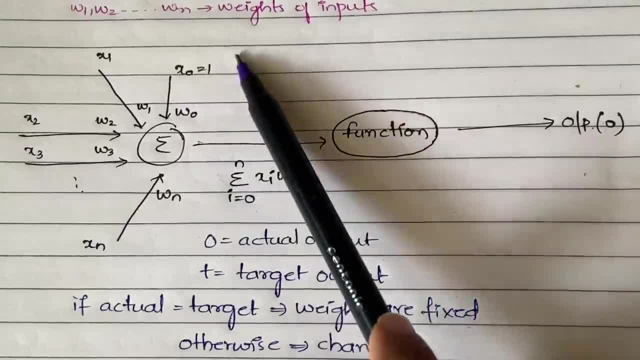 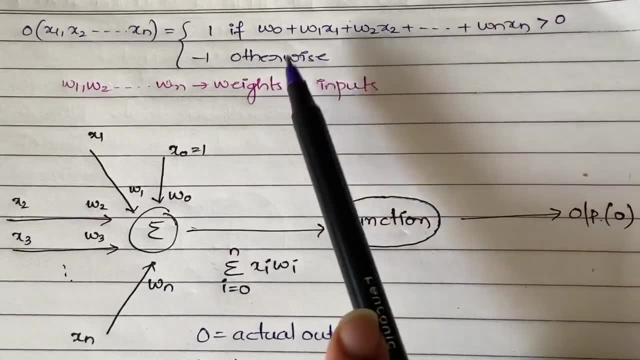 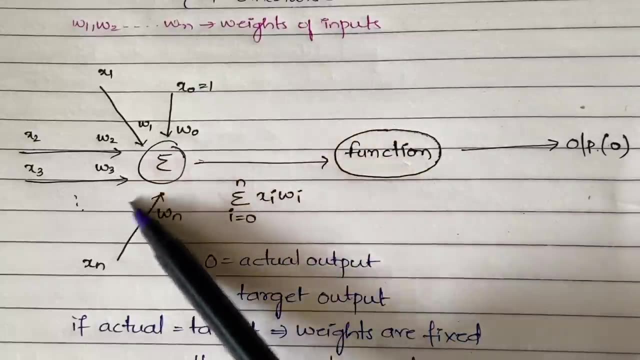 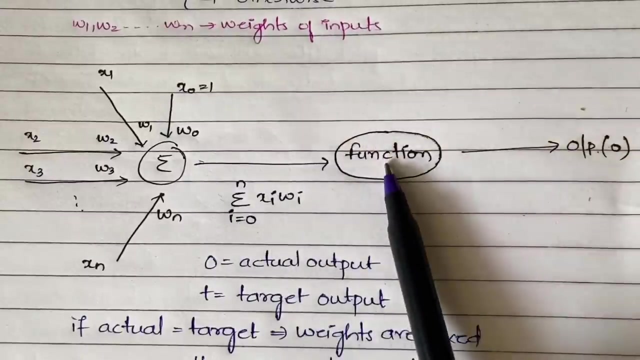 And its weight. X0 is equal to one and W0.. Okay, since X0 is equal to one, So X0 times W0 will become one into W0, which is not, which is nothing but W0. That is what we have taken here: W0.. Okay, so we will be giving all the inputs to the summation function. What the summation function will do, it will add up all the inputs, right? So it will add up all the inputs and whatever the result is obtained, that will be sent to the function, right? This is the perceptron training rule. Okay, this is different: The one minus one output. 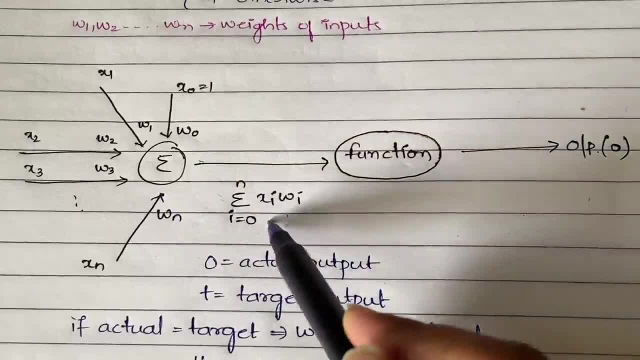 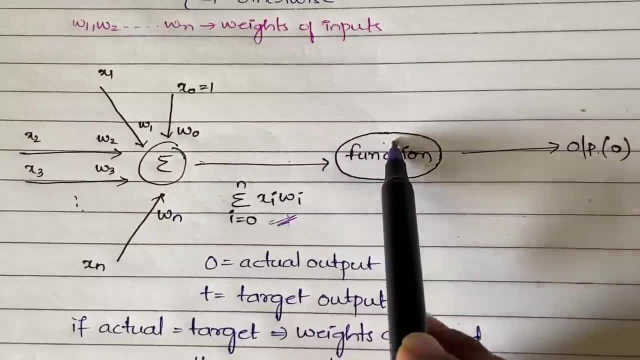 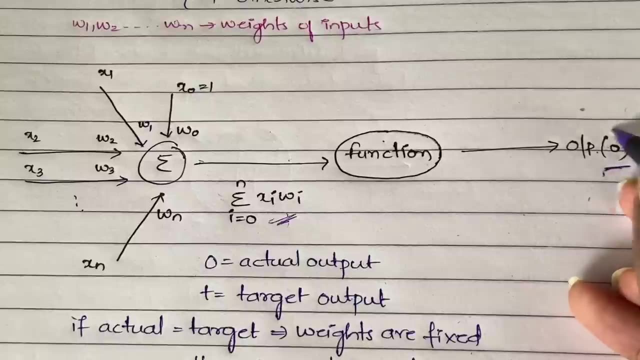 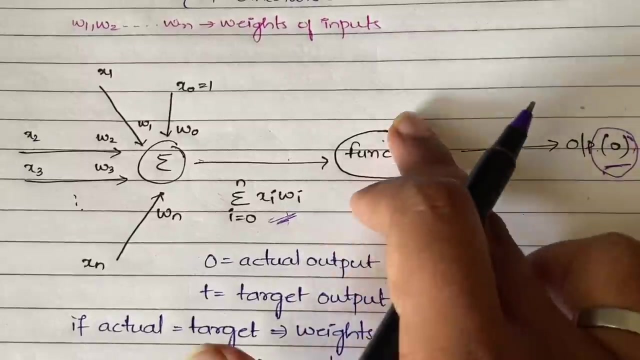 The output is different, right? So one minus one output you will get for this, right. And now, once the output is obtained, that will be sent into the activation function. What activation function will do? it will generate the output, as we know, right, And the output is represented by O here. O is nothing but the actual output, Okay, and T is nothing but the target output. Who will generate this actual output? the function will tell: generate the actual output and what is the target output? whatever target output. 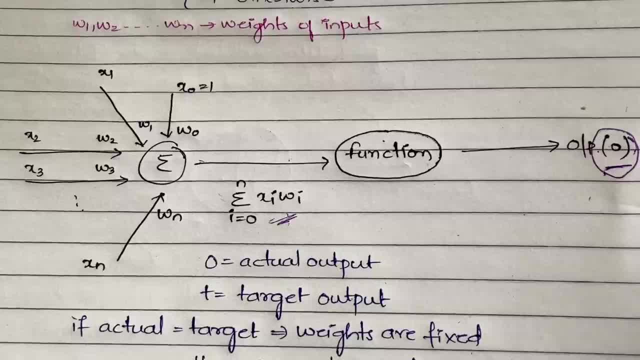 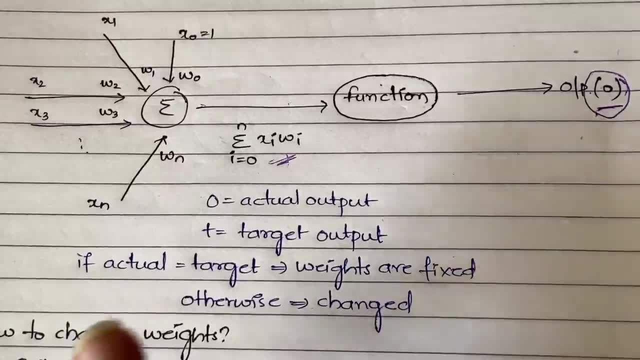 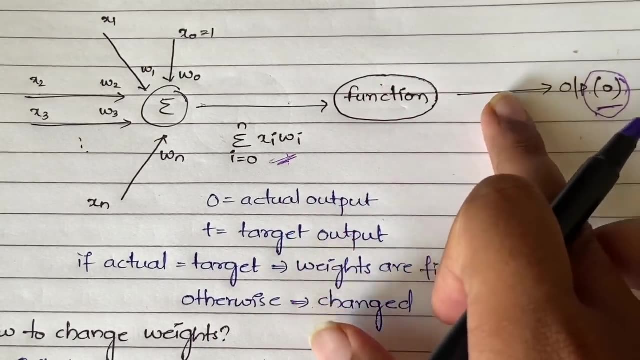 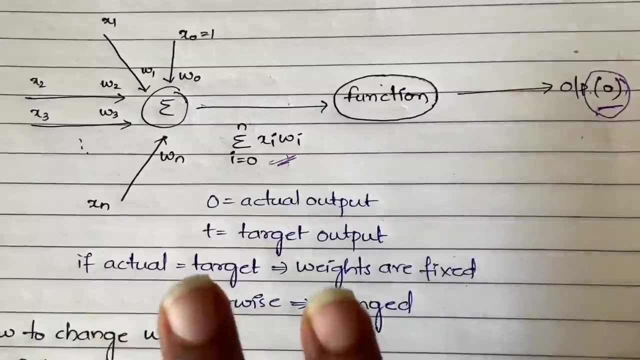 We are expecting, expecting output, actual output also, you can say So. whatever the target output we are expecting, that is represented by T. Okay now, if the actual output that we have obtained out of target function is equal to the sorry, out of activation function is equal to the target output, then the weights are fixed. That means these weights, W0 to Wn, are finalized. Okay, so W1,, W3, whatever weights you have taken initially, you can fix them, you can finalize them. 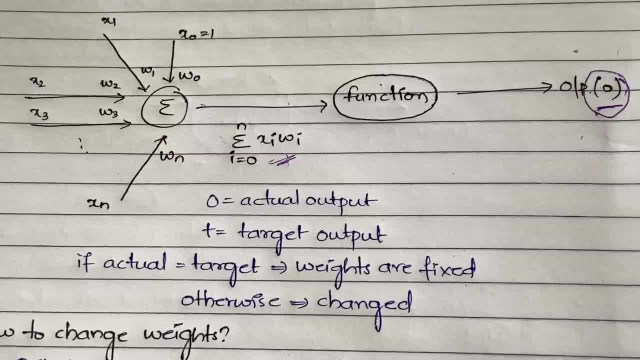 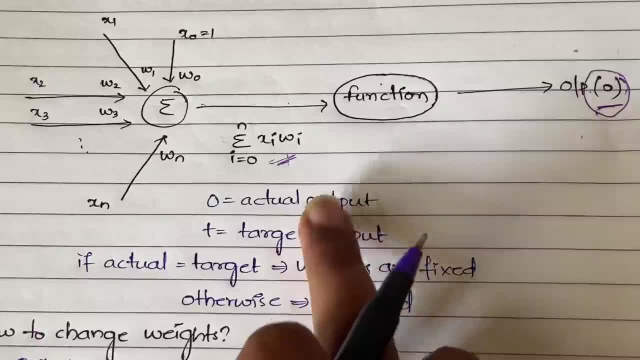 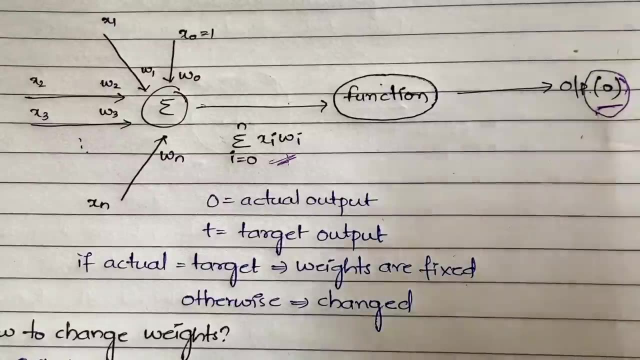 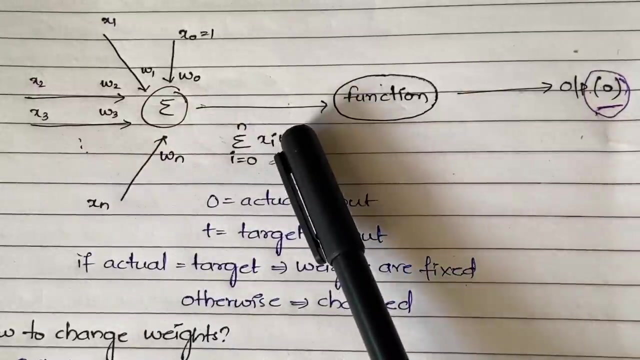 And you can train the perceptron based on those rules. only, those weights only. But if the weights are not equal, then you sorry, if the actual output and the target output are not equal, then you need to change the weights. How you will change the weights, you have a small formula for that. I will tell you that also, don't worry. Okay, so a clear, be clear on this. I am telling you once again: the summation function will generate a linear combination of the inputs and that will be sent into the activation function and activation function will generate an output. 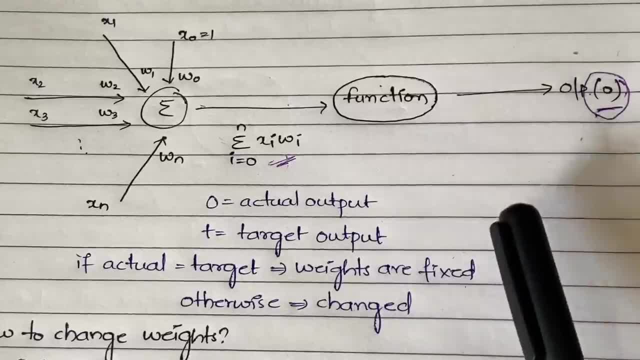 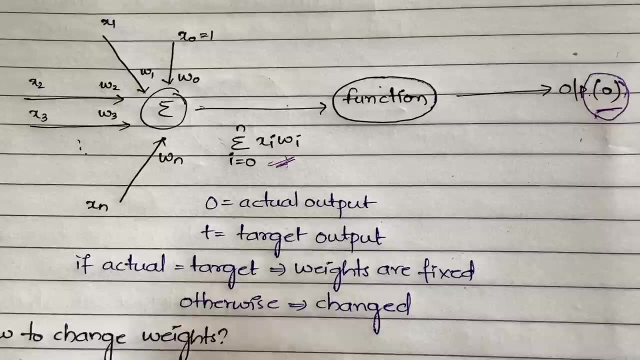 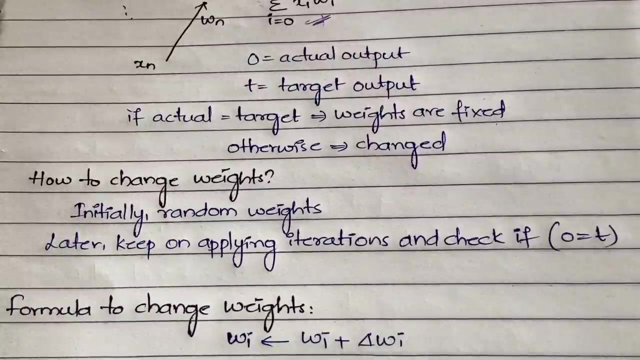 Which is nothing but the actual output. And we are already having target output with that, That actual output which we have obtained and the target output, both of them are compared against each other. If both of them are equal, the initial weights which we have taken, they are fixed. If they are not equal, we need to change the weights. And how we have to change the weights. I will show you See how to change the weights. First, what you have to do: initially, you need to pick up some random weights- Okay, something of your choice, You can take any weight- And you need to do this entire step. 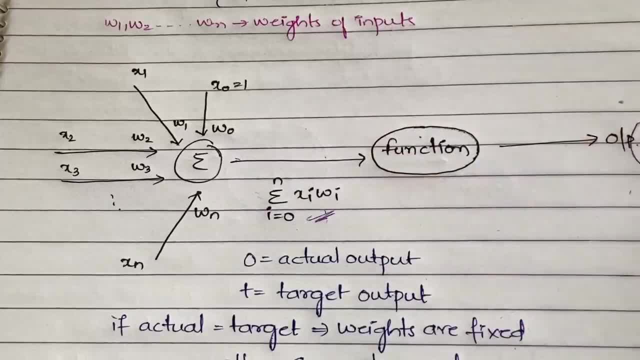 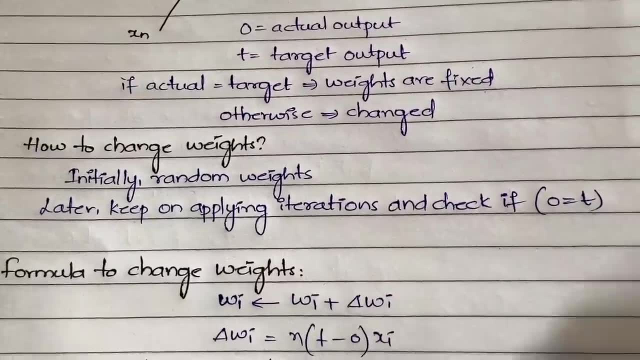 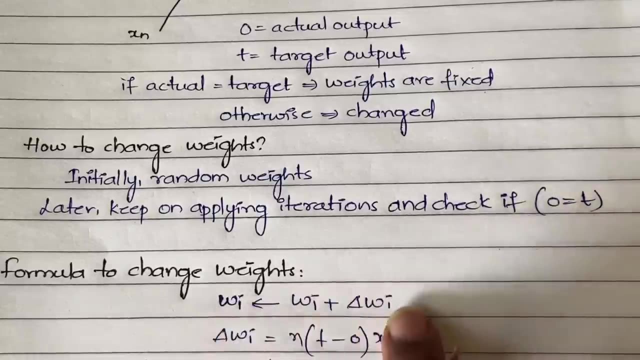 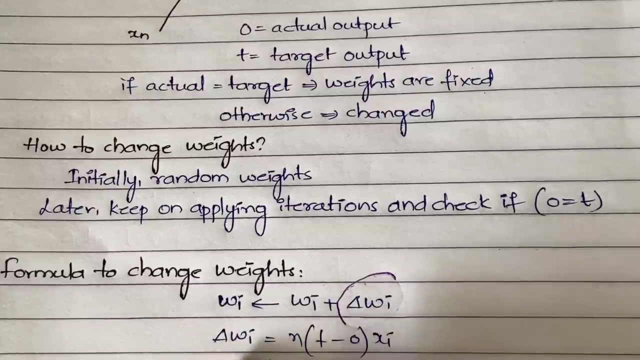 Okay, like summation, multiplying the respective weight summation function, and all You need to do. Once done, you need to check, Right? If they are not equal, then what you have to do, you need to use this formula: WI is equal to WI plus delta WI, So initially it is WI, Right? You need to add a small value, which is called as delta WI, to it in order to change its value, Right? And how do you get delta WI N multiplied with T minus O times XI. So here, what is N? 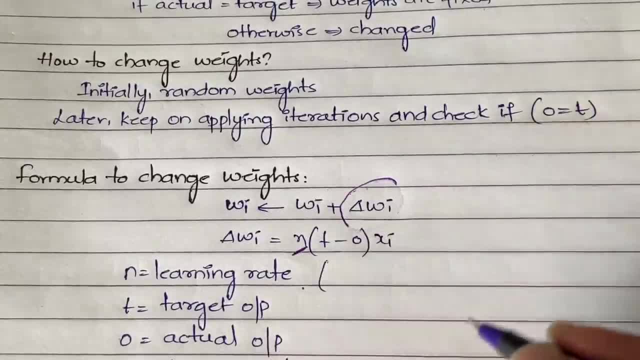 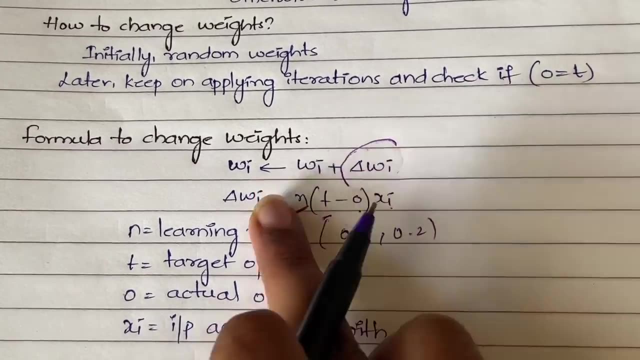 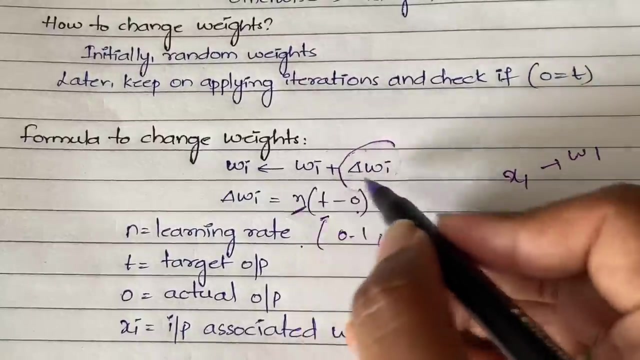 N is nothing but learning rate. It is usually set to a small value like 0.1 or 0.2. like that You will have a small constant for learning rate. Okay, And here T is the target output, O is the actual output And XI is the input associated with this weight, WI. So XI, X1 has W1. Right And X2 has W2. Right. So whatever the input is associated with this, WI will be taken here. Suppose, if it is W1, you need to take X1. 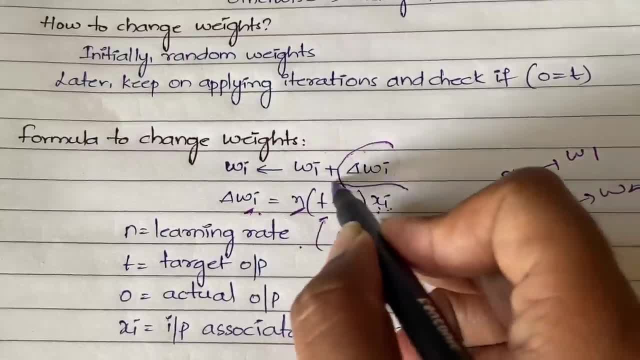 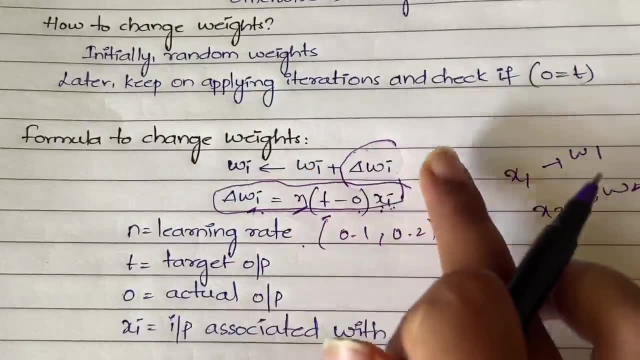 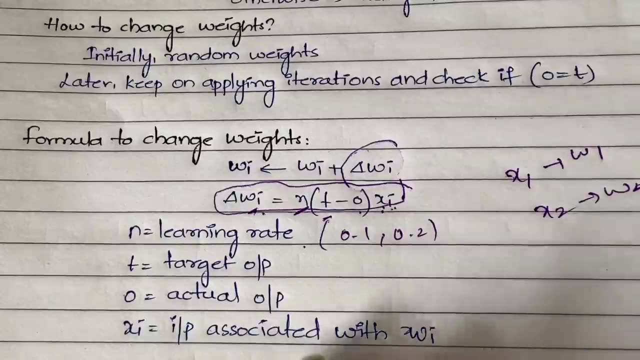 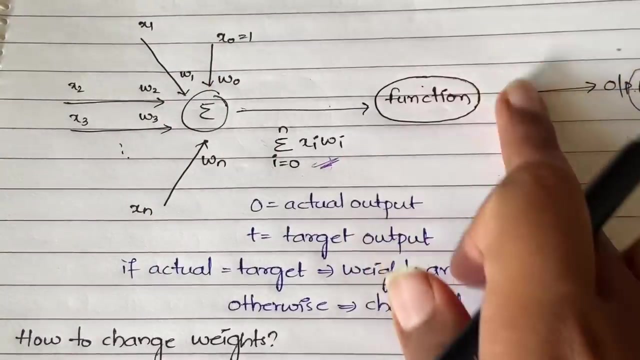 If it is W2, you need to take X2.. Okay, So this is how you calculate the delta WI and whatever the delta WI that you have obtained, that you will be adding to the existing WI. That is, you will be adding that to the existing weight you are having And then, like that, you need to increment for each and every weight How many weights you are having. Suppose, if you are having four weights here, then you need to increment all the four weights And again you need to do the function And again you need to check whether output- actual output- is equal to target output or not. 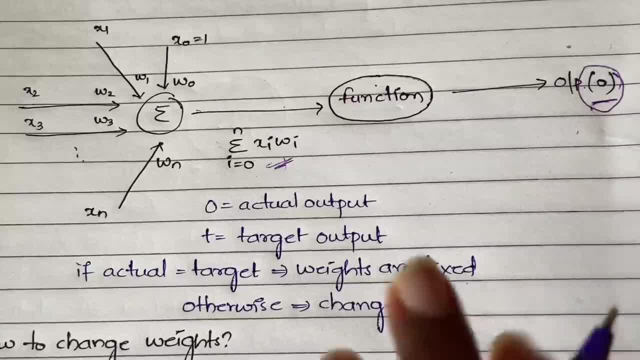 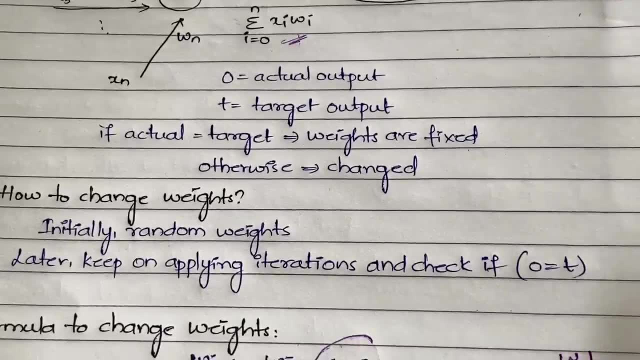 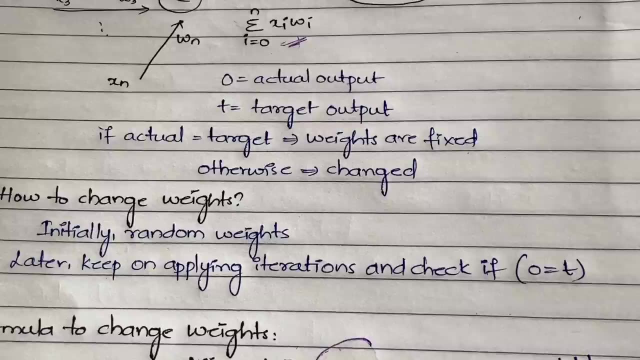 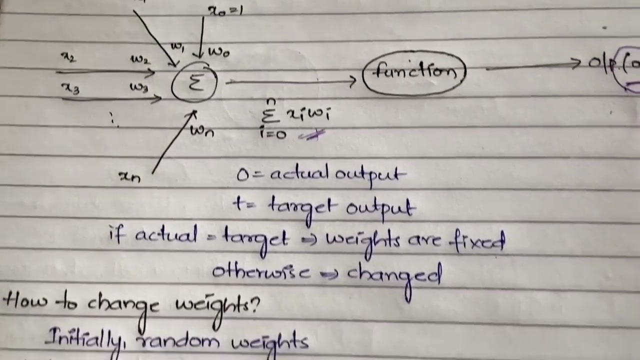 If they are equal, okay, well and done. If they are not equal, again, what you have to do Again change the weights. So, like that, you should do several increments until and unless you get output. actual output is equal to target output, Okay. Once you are done, you need to finalize upon weights. Right, You need to finalize upon weights, and they are the final weights that you can use to train up your perceptron. Okay, So this is how perceptron training rule goes on. First, you need to calculate the actual output, And that actual output is to be.